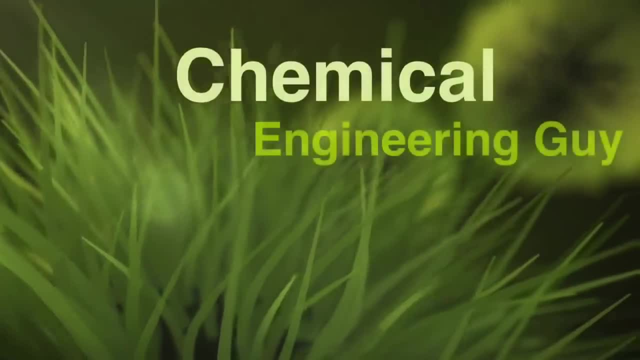 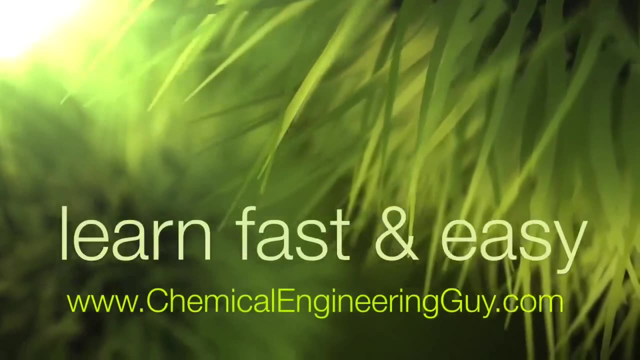 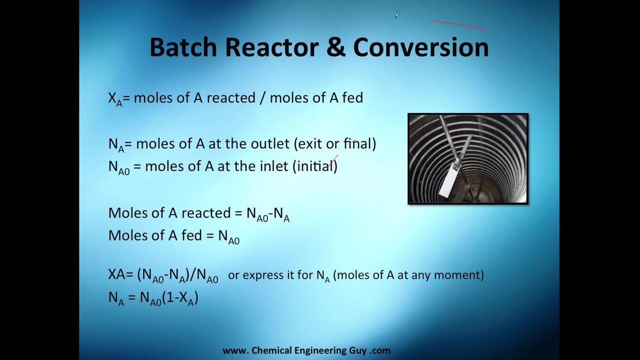 So we've seen before something about conversion and I told you that we're going to apply it to our design equation. so the first one I want you to show is the batch reactor, which is not a continuous flow. it's actually a unsteady or transient process. actually, it's a batch process, so it's the only one which 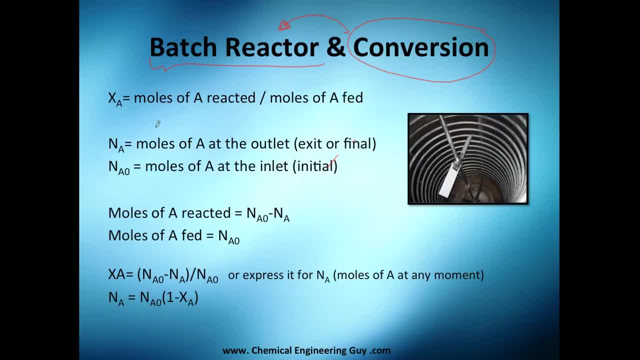 is going to be different, so pay a lot of attention here now. by definition, this is conversion of A. it's the moles of A being reacted per moles of A being fed. okay, the case in batch, or at least in the batch reactor, we're going to have N. 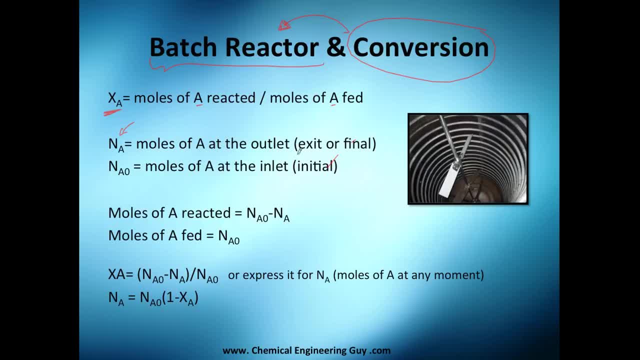 of A, which are the moles of A at the outlet or at the ending or at the final step, and I got N of A zero, which are the moles of A at the inlet, or the initial amount of moles of A. normally, by definition, N of A initial is bigger than 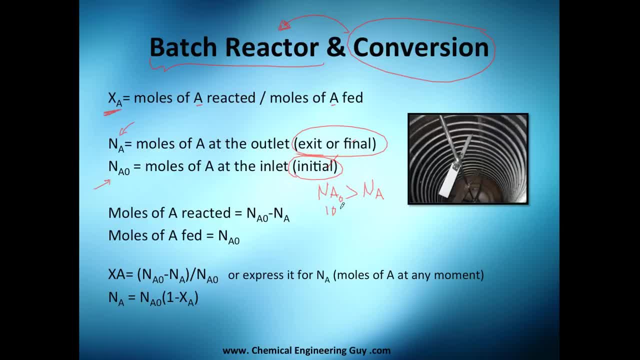 the final amount because you're reacting. so you have 100 moles and you react. I don't know X quantity. you're going to have less than 100 moles. let's say you're going to have at the ending 20 moles of A or, best case scenario, you turn. 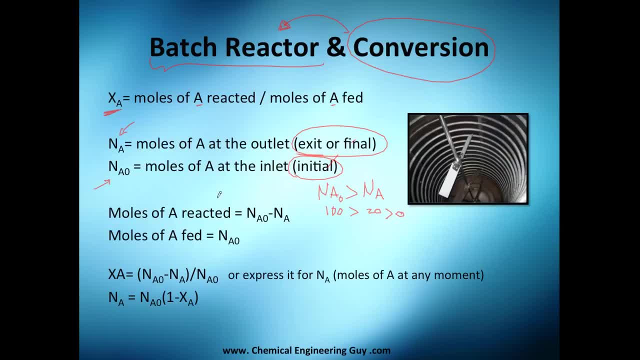 everything to the product. so you got zero. now pay attention in this equation, what are the moles of A being reacted? well, the moles of A are the initial amount, which is the 100, in this case, minus the final amount, which will be, let's say, 20. so I used to have 100 moles of A at the 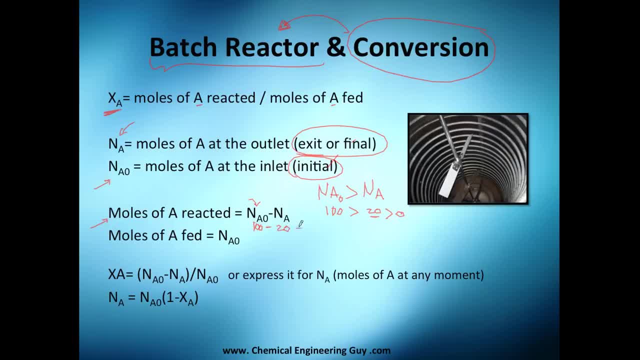 beginning and I still have 20 moles. at the ending that 80 moles disappeared. what does that mean? that 80 moles just reacted. so that's the moles of A being reacted, which is this number right here. the moles of A being fed is way easier. it's essentially just the initial amount of A. 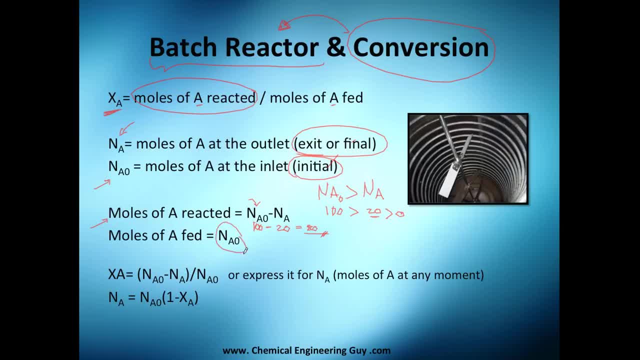 which is Na0. so now you got your definition, let's say, let's go back to here. let's go back here. x of A equals the total amount of moles being reacted, which is this here we told you. right now it's this one here divided by: 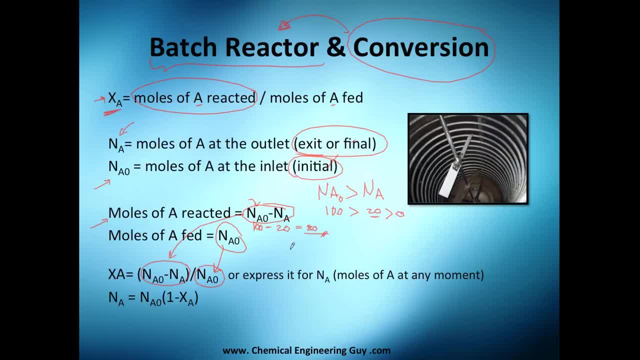 the initial amount of being fed, which is here, okay, and I don't think that this is useful. but the other, let's say, when you do it, sometimes you want to know the amount of A at any moment. well, of course, you're going to have it, depending. 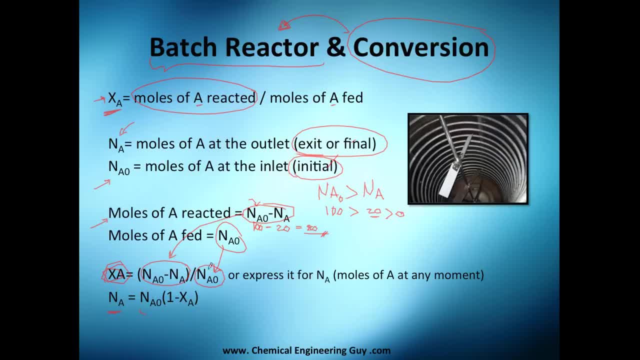 이번에 noи olduğ heart我們или dari A ticked by здесь. okay, so now I think it's going to be happening. depends데 otra vez naí식 on the conversion. so you got them. i just go and find out or solve for this one, you get this one. 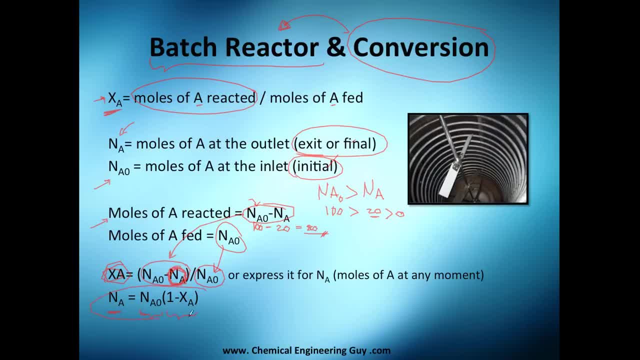 here, times one minus x of a. this one is also very useful. actually is the one that we are going to be using the most. but don't worry, it's the same equation, it's just mathematics. i just move this one here and this one minus this one, divided by the negative, you get this equation so perfect we. 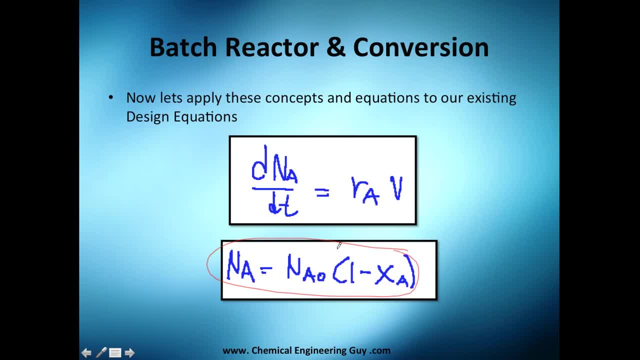 got our, let's say, conversion equation in terms of moles being fed and moles at any moment, and we got our design equation. if you don't know where i got this, you or you have no idea- go to the batch section. i got a class in which we use this molar balance equation and we got this. so what i'm going? 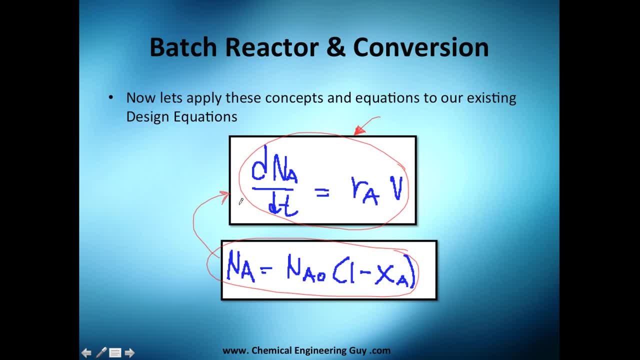 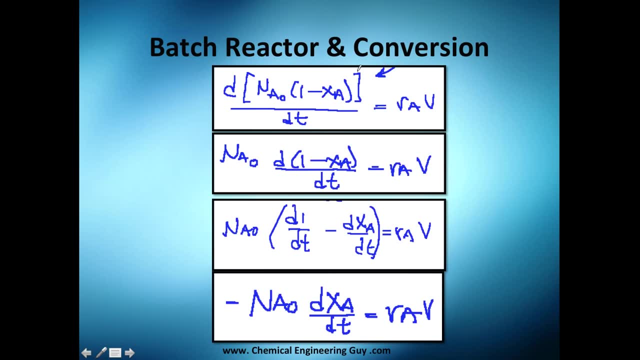 to do essentially is to use this equation and substitute it here. essentially, this right here, i'm going to put it here so you can see i only change this part here. and since the total amount of moles being fed at the beginning is a constant, so that's a value that's not moving, i can take it away from the derivative. 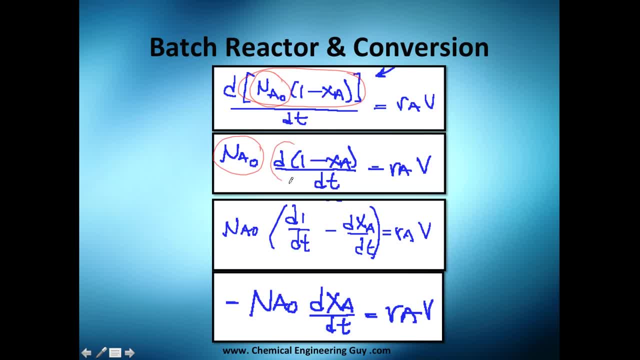 and if you know a little bit of derivatives, i can split this into two derivatives: this one, derivative of one, with respect of time, and the negative of the derivative of x of a with respect of time. probably you know this is a constant because the derivative of one is constant. 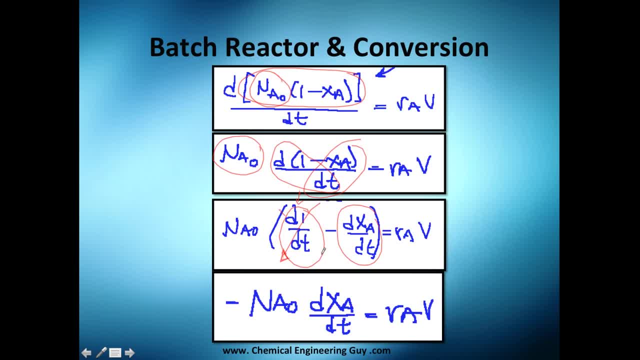 or zero, actually zero, not a constant. it's zero, this is zero, and i just got this negative out and multiply it times n of a, or initial amount of moles, a. now, just to let you know. the right side is exactly left alone. you have no actions. we did not do anything there. 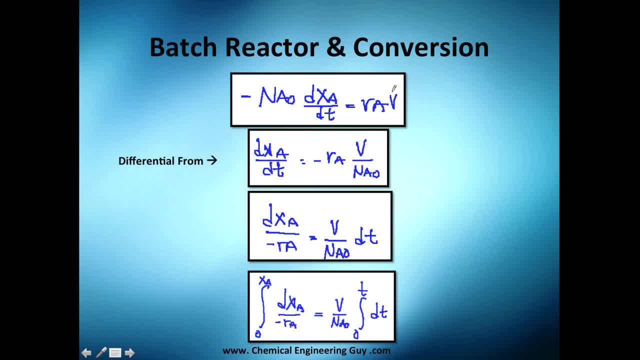 so now we got these equations, what i will do is the differential form. i want to get this derivative in the left side and i change this one here. and since you know, i love having this minus r of a, which is the rate of reaction, reaction of a and we are very happy. we have volume, we have 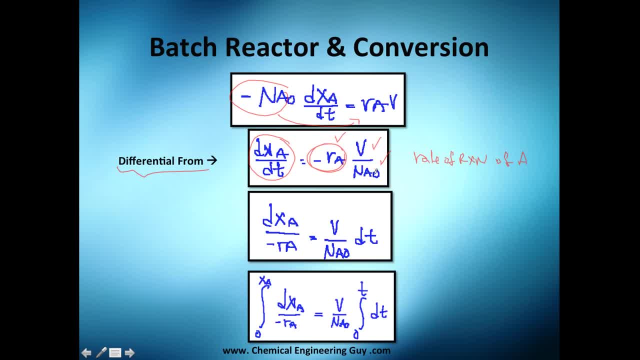 initial amount of a being fed. we got this rate of reaction and this derivative, So I like it. I will learn this one. Many people like to develop it and learn the final equation, but that's not that good of an idea because maybe you get this volume. 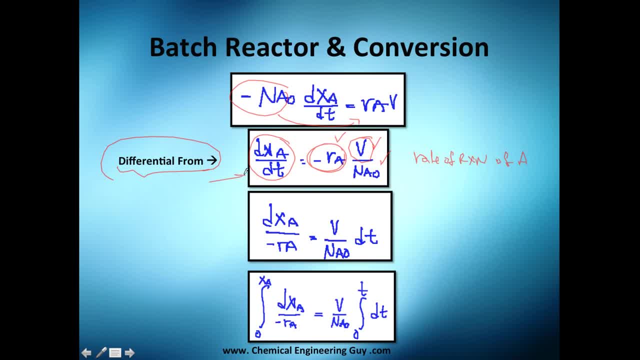 that changes with time or I don't know. I just prefer to have it like this and develop it by myself. So let's develop it, Let's do a little bit map. So the first thing I want to do is to change the rate of reaction to here, because it's dependent on the conversion. 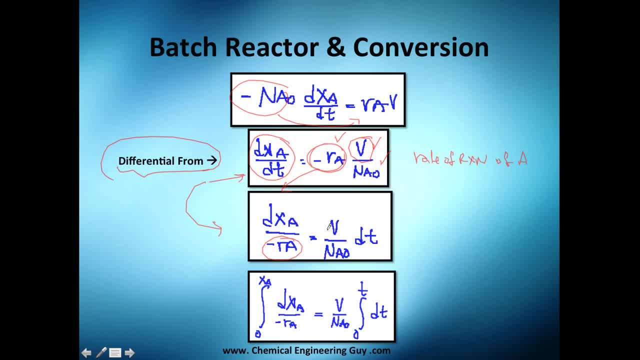 It's very important, guys, that you know that the rate of reaction depends on the conversion. You got X of A with 0 and X of A at 30% and X of A of 50%. Probably you're going to have different rates of reactions. So this rate, X1 is not the same as X2 and it's not the 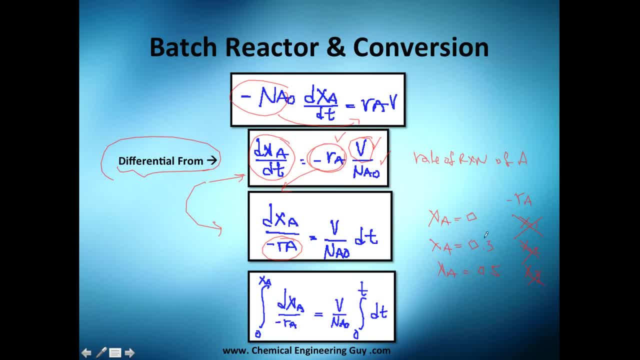 same as X3. So please, guys, be sure to know that rate of reaction. It depends on conversion. Now I change the differential of time, I change it here, And since this is a constant, I can just drop it away from the integral. I integrate this left. 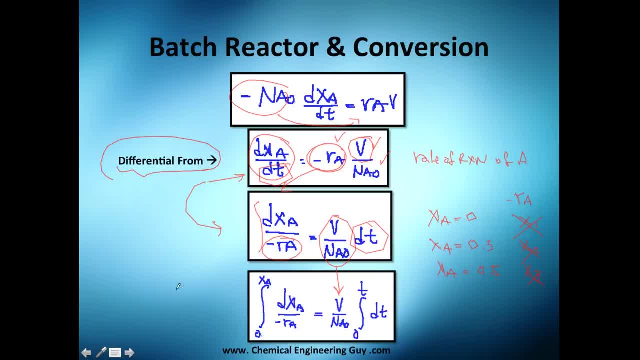 side, from 0 to my final conversion. Why 0? Because that's my initial quantity At the beginning of time. I have 0 conversion. I have 0 time 0 conversion And at time or any time, I have my conversion. 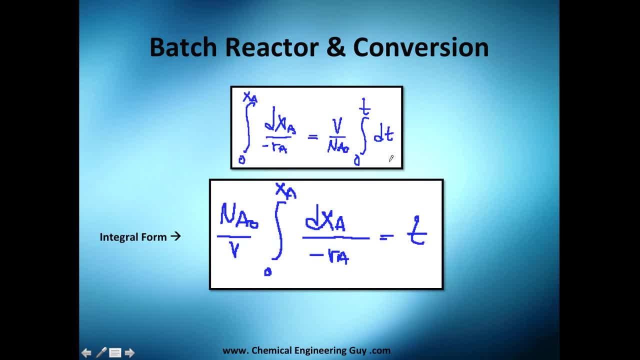 So we have. this is exactly the same as before. Now we're going to do this, This part, right here. I'm going to send it multiplying to this side. So that's why this one goes up and this one goes down. Now the limits stay the same: 0 to conversion. I cannot develop this because 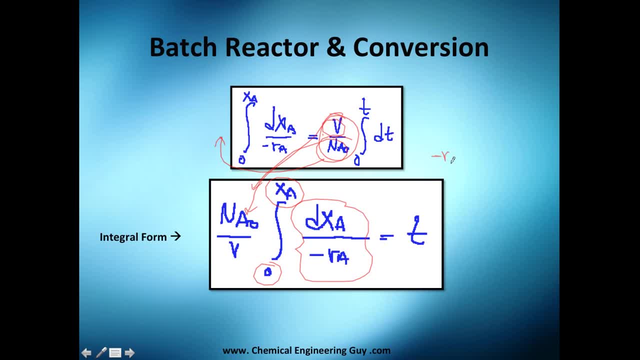 I don't have an expression for the rate of reaction. If they tell me rate of reaction of A is 1, well, yes, I could integrate very easily If they tell me that the rate of reaction is 1 divided by the concentration of A is 1.. 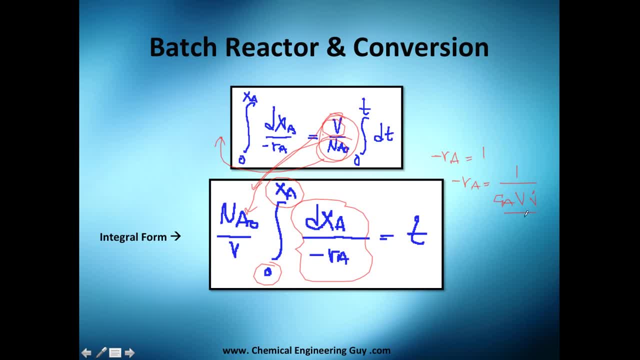 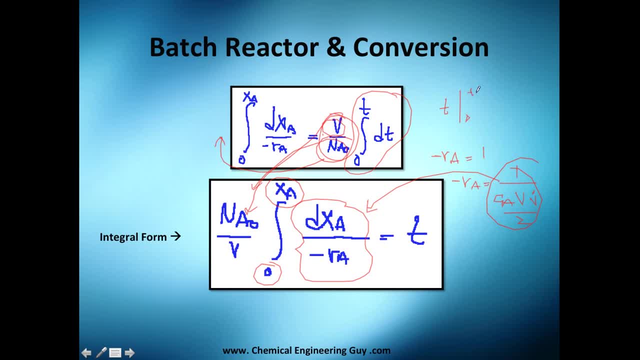 of 1 is t. I need to value it in these two values, which is t minus 0, which is t. So I got this equation on time. So this is my final equation. if you really want it like this, I don't recommend it. I. 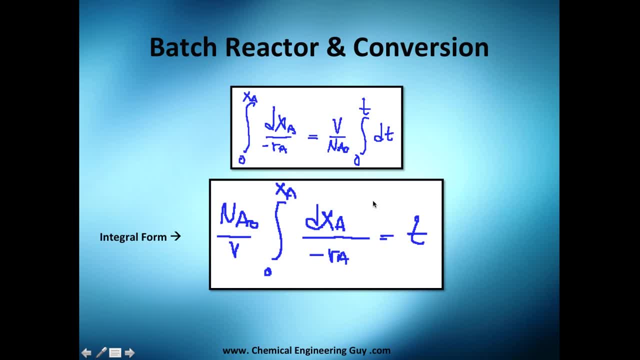 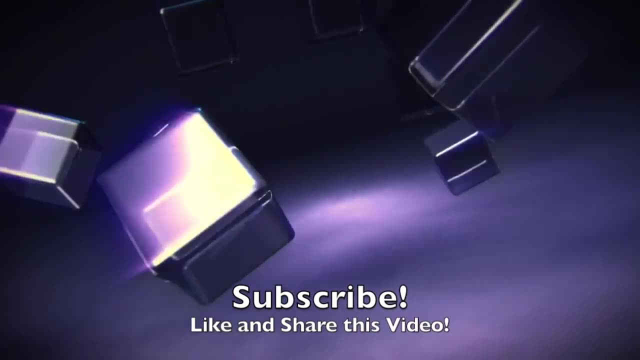 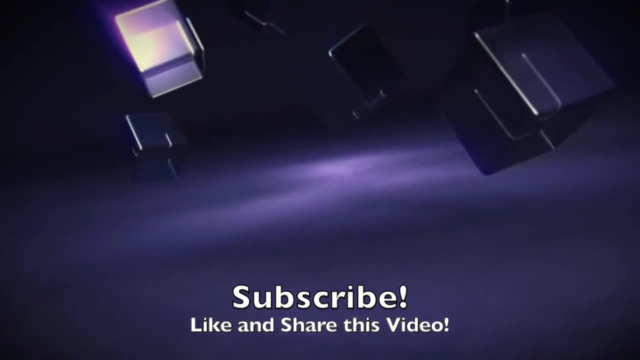 prefer it in differential form, But it's up to you, guys. And this was how we change the batch reactor design equation in terms of conversion. See you in the other videos. What's up, guys? It's me, Chemical Engineering Guy. So if you liked the video, why don't you? 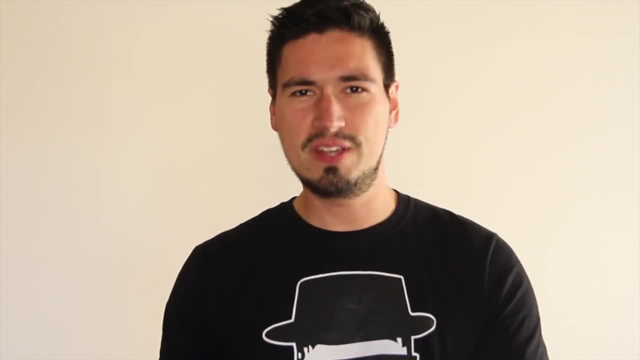 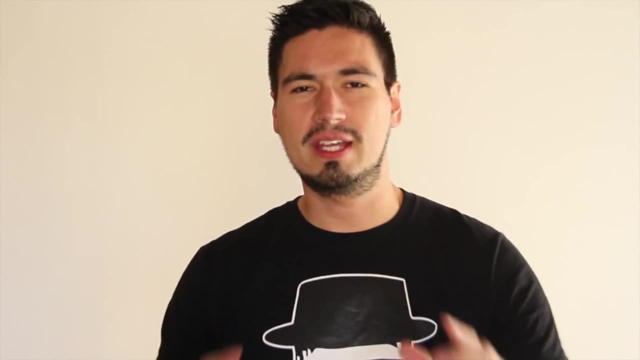 push the like button. It really helps me to know if you're liking the videos or if I should be changing something or I should be adding something, taking out content, whatever. Also, sharing is caring. So if you got any kind of friends, teachers, colleagues or whatever, 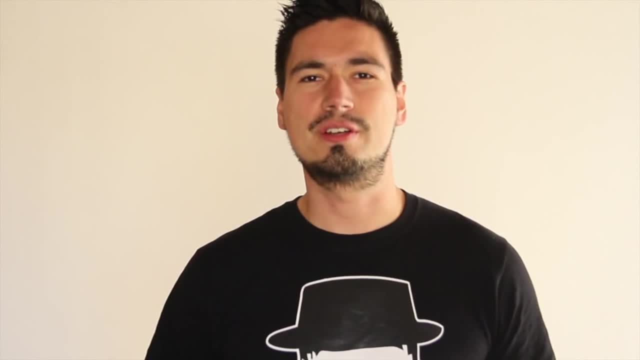 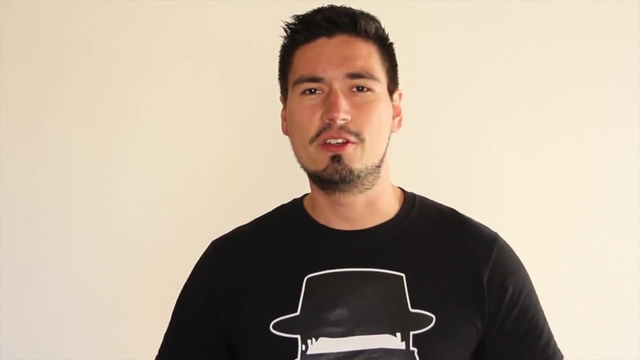 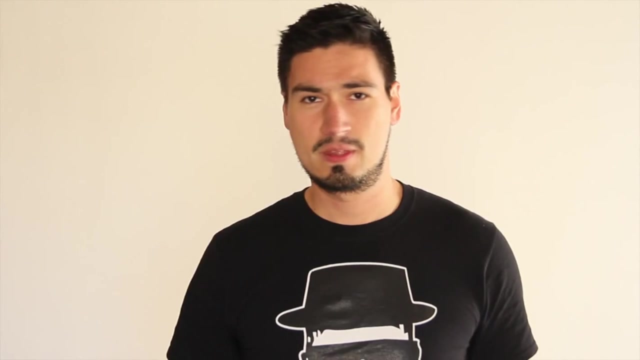 kind of person that might be interested in this type of content. why not share it? Sharing helps our community to grow faster- in members and in content. If you want to keep track of my activity, videos, book loads, experiments, playlists- whatever content I'm getting on YouTube- be sure to click the subscribe button. Subscribing.